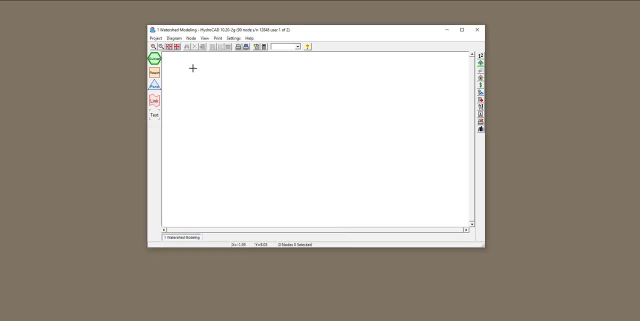 Open and, yes, I want to create a new project. So now you can see some of these buttons and bars are activated over here. I'm going to talk about all of these as we go on through this tutorial series. All right, but in order to do watershed modeling, we need to have a watershed. 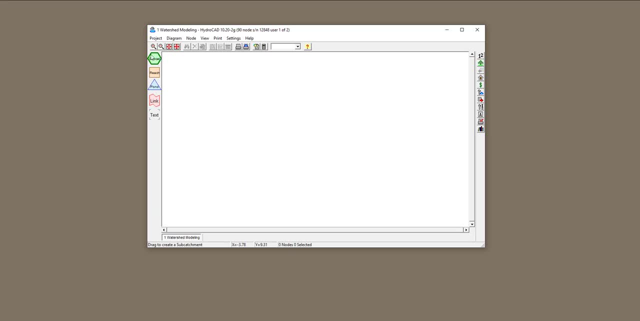 or a subbasin. So when you take a look at this green button over here, it says subcatchment. I'm going to drag the subcatchment into the white screen over here and this would be one subbasin, subbasin one or subcatchment one, right, If you right click on it, you can edit that and change. 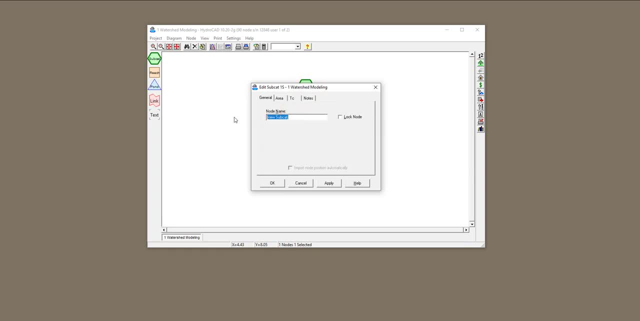 the name of this node or subcatchment into whatever you want to. I'm going to change it to subbasin one and click okay, Okay, so now I have subbasin one. There are lots of things that you can change in, like area, time of concentration, so on and so forth, But first of all we need to. 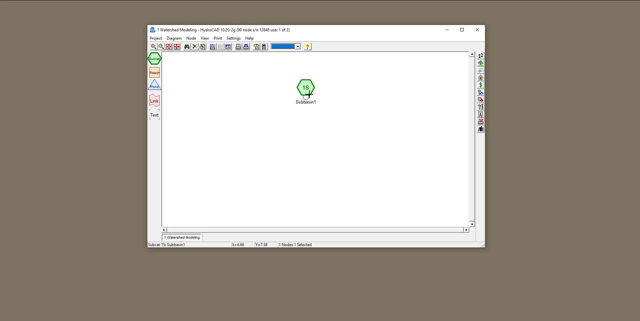 realize what is the method that HydroCAD is using for calculating surface runoff. Take a look at this calculator over here. This is called calculation settings. When you click on that, it will tell you that the runoff method that HydroCAD is using right now is SCS curve number method, based on 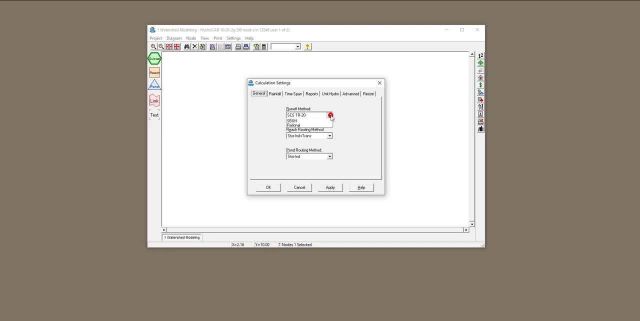 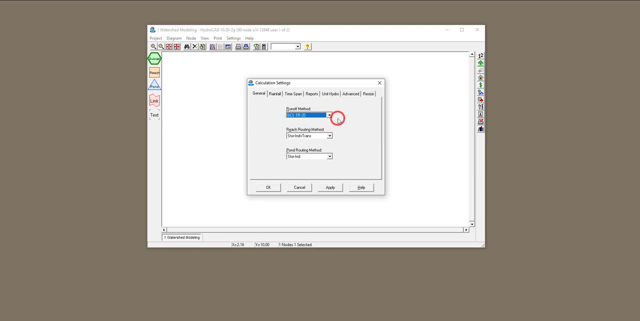 keep it as SCS curve number. So that depends on what method you want to use to model the runoff in your subbasin. I'm going to keep it as SCS curve number method. Okay, so now I'm going to right click on my subbasin and click on edit. This will allow me to define this watershed. So first of 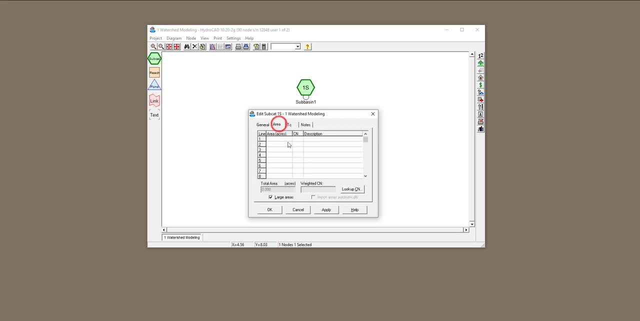 all, again, we have a name for it. Then I'm going to go over area The area. you can see that the units for area are in acres. What if you want to define this watershed in acres? Well, you can change the units. Let's close this. If you want to change the units of input and output, you can. 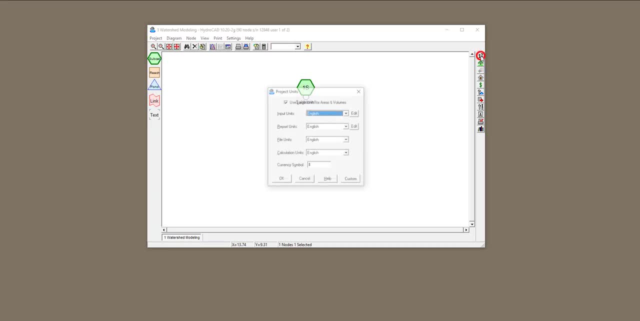 simply go to this vertical ribbon over here and click on set measurement units and change the units from English to metric and so on and so forth. For this specific problem, I'm going to keep the units as English. All right, let's right click on subbasin and edit. go back to the area. 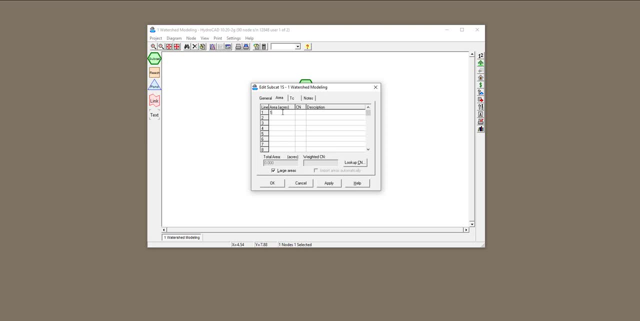 I am going to consider that I have one area and I'm going to keep the units as English. So I'm going to go to the area and I'm going to say that I have one acre of maybe residential areas. So now I need to find the curve number for this, If you remember, in order to find curve number. 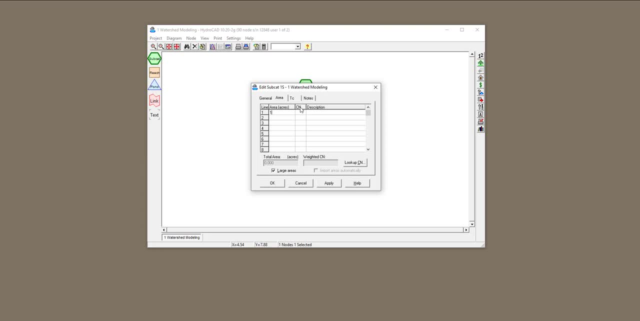 you need to go to the NRCS manuals or TR20 manuals and find the value of curve number based on land use, hydrologic condition and soil type. right. But the good thing about HydroCat is if you double click over here, this is going to open up the value of the curve number. So if you double click over, 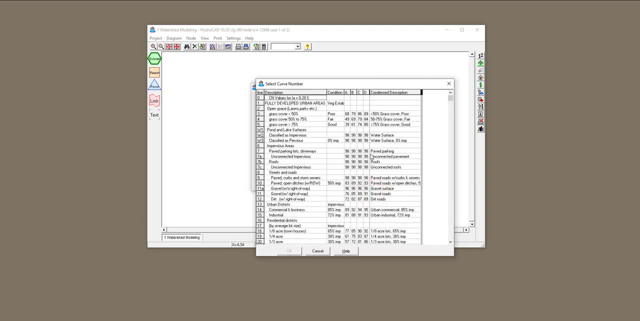 here. this is going to open the curve number table for you. So what you need to do over here is just go through all of these and find what you want over here. Okay, so take a look at this. We have. I said that I want to consider residential district and my area is one acre. I'm going to 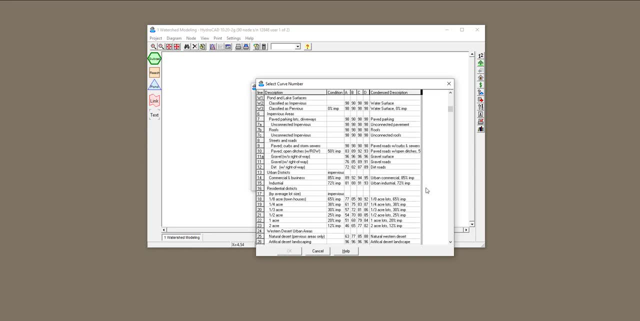 consider 20% impervious, okay? And then if you go up here, you can see the soil types, soil hydrogroups A, B, C, D, I, M, Z and Z. So I'm going to go up here and I'm going to go to the area and I'm going to 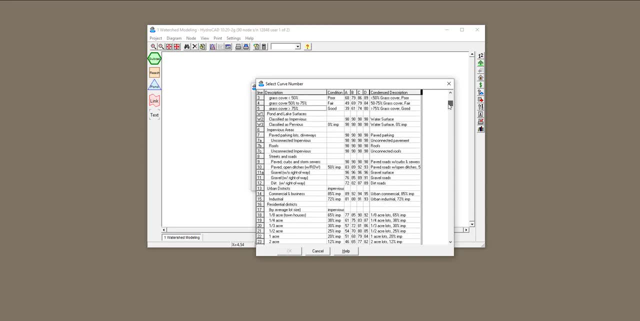 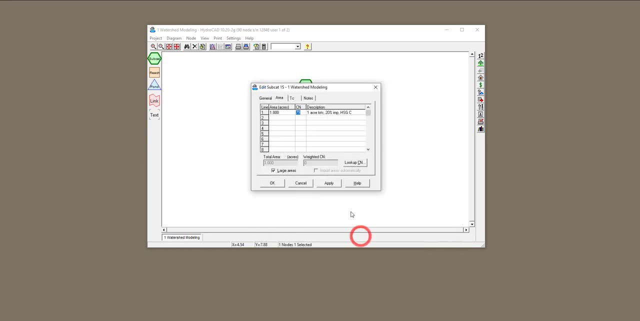 consider the hydro group: soil hydrogroup of type C. So it would be right over here. So when you click on it, when you double click on it, it will automatically choose that curve number for you and it gives you a description. If you want to edit the description, you can always add to this description. 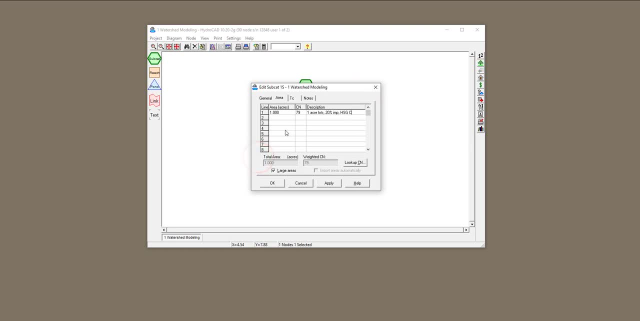 to make it more descriptive. What if you have several areas? I'm going to talk about this in the next section of this video. Right now, let's say that we know that we have a residential area one acre and curve number is 79, and that 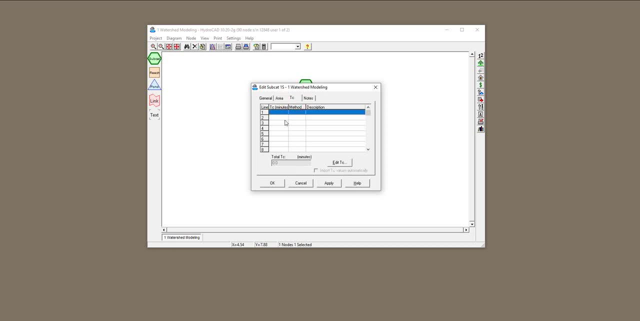 would be it. Next, we need to talk about time of concentration. Again, there are different methods to calculate time of concentration, And what is time of concentration? Time of concentration is the time that it takes for a drop of water to travel from the furthest hydraulically furthest. 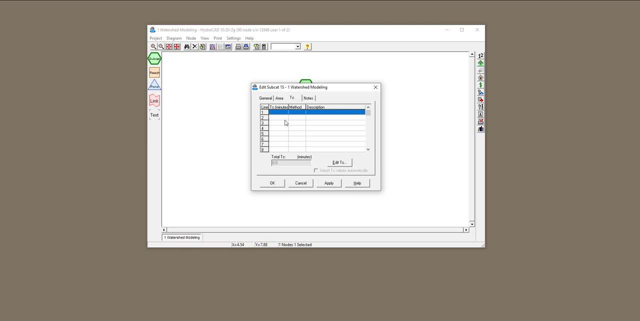 point of the watershed to the outlet of the watershed. So this is the physical minute meaning of time of concentration And it is- you need to put it in minutes, But if you know the time of concentration, so if you double click over here, you will see that there are different methodologies. 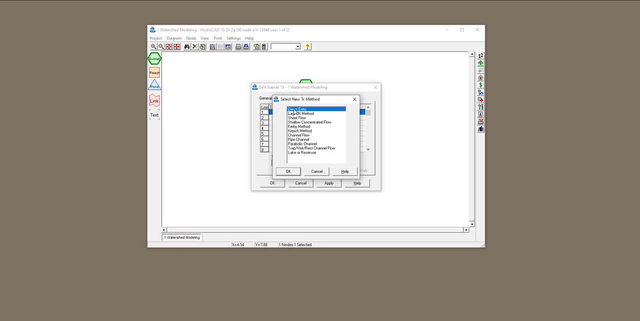 for calculating time of concentration. If you know time of concentration, you can click on direct entry and then add a description that this is the value that I have based on this report or that report or someone told me, and then input the value of time of concentration. In my case it's. 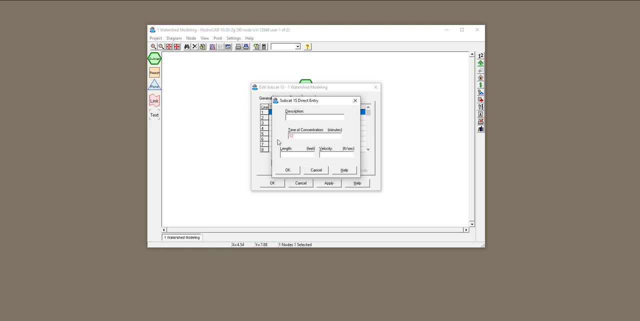 going to be 12 minutes. If you know the length of the length that water travels and the velocity, that's good. If you don't know it, it's optional. You don't have to input it over here And I'm going to click. 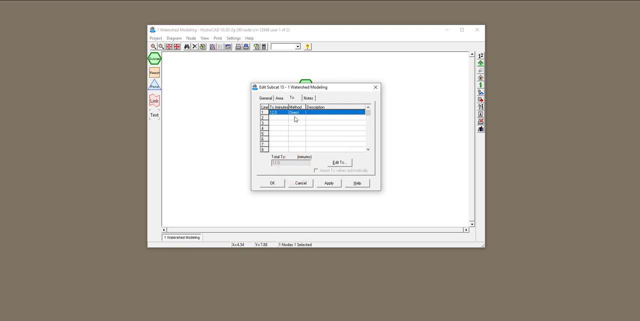 on. OK, You're going to ask me what if I want to use a different methodology for time of concentration, and that would be the topic for the next section of this video. So my total time of concentration is 12 minutes And now that I have this, I can go to the notes And if I want to add a note, 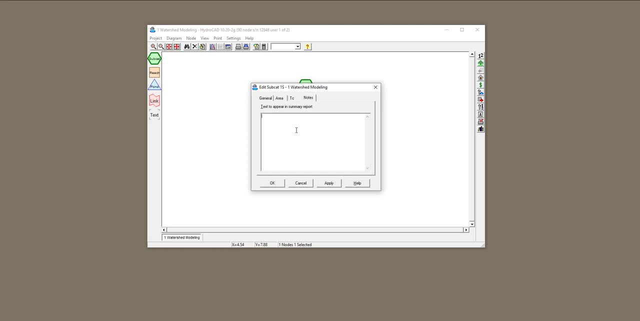 somewhere to this, which will be added to the summary report, I can put it over here. All right, Then I'm going to click over here And now, if I right click and then edit, you will see that all the information that I input is saved over here. Perfect, So the watershed parameters. 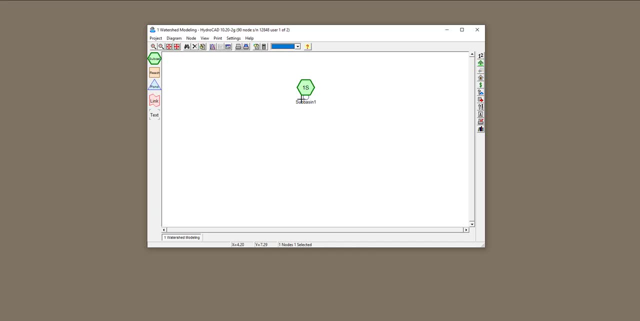 characteristics are there. Now we need a rainfall. That rainfall is going to fall on this watershed and it's going to create a hydrograph, And we are going to see the hydrograph at the outlet of the watershed. But how do we create that rainfall? So, if you want to create 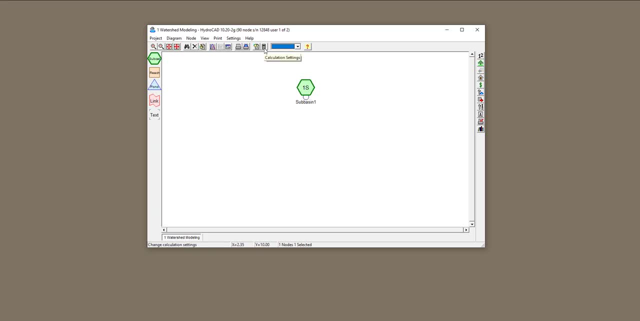 a rainfall, we need to go over calculation settings. I'm going to click on calculation settings and there's a tab called rainfall. In this rainfall you can define your rainfall depth over here And normally rainfall depth is defined based on NOAA Atlas 14.. So you can define a depth for that. 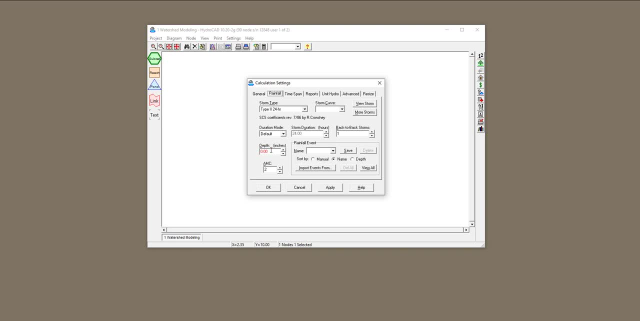 So you can define a depth for this, You can define a depth for the rainfall depth. You can define a depth for that for a specific return period and duration. Another thing that you can do: actually, you can import different rainfall events over here. 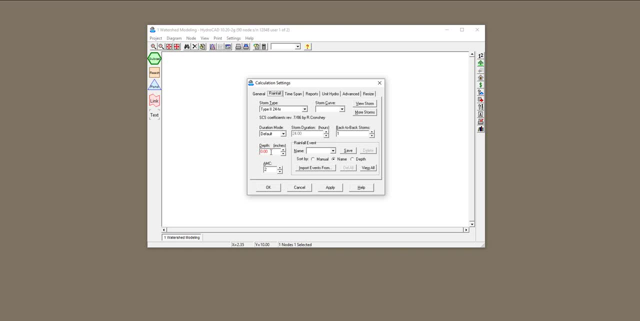 But for this part of the video we want to keep it as simple as possible. In the next sections of this video we're going to add to it. So let's call the depth. let's actually say that the depth of rainfall that we are going to receive is going to be 2.5 inches. 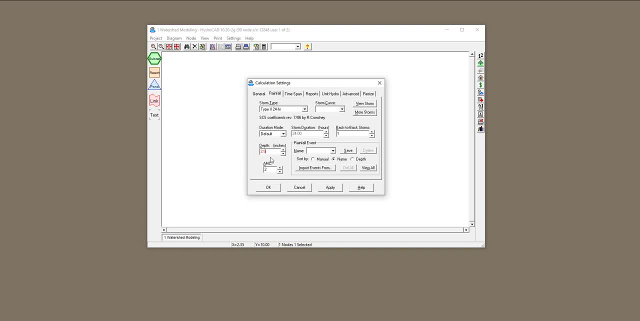 Okay, so this is the total depth of rainfall, but we want our rainfall to be distributed over time. A very common distribution that water resources engineers use is type two, 24 hour distribution. Well, type two refers to the location that you are in. 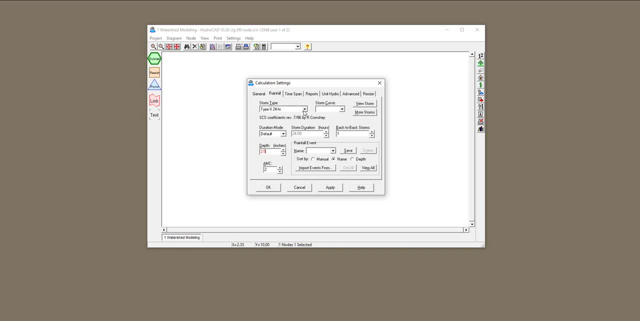 Because I know I am in the United States, in the Midwest, so I need to use type two. If you're in different areas, you might need to use type three or type one If you, instead of having 24 hour distribution, you want 12 hour or six hour. 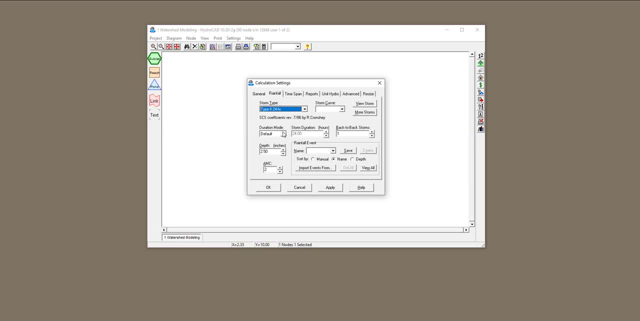 you can change these as well, Okay, and then if you want to rescale this, let's say if you want a two hour rainfall, you can click here and click on scale and then change this 24 hours to two hour. Okay, but right now I want to go with the default. 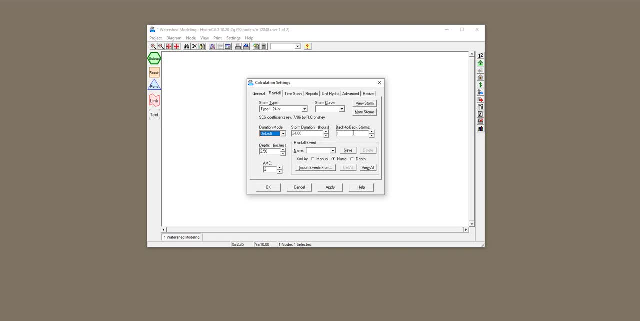 Okay, you also have the option of having back to back storm. Let's say, instead of one rainfall, I want to have two rainfalls, So you can change this to two. It will be two. back to back storm. Back to back rainfall events. 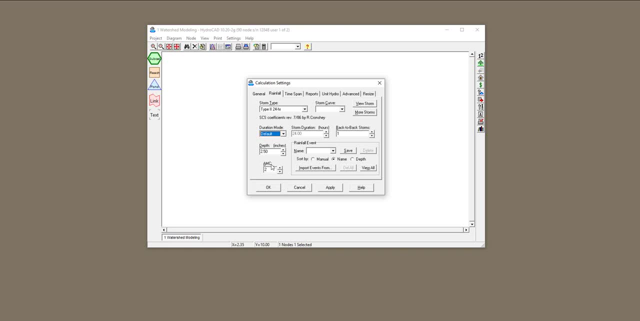 And AMC is the antecedent moisture content. So two and AMC is the antecedent moisture content of the soil. Two means that we have the average condition. It's not dry and it's not wet. You can change it to one and three. 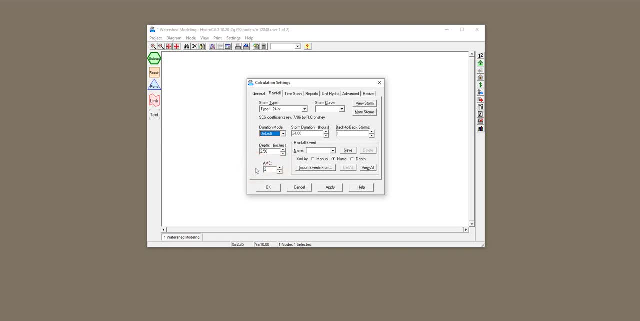 depending on if your condition is dry or wet. If the antecedent condition of the soil is dry or wet, Again, I'm going to keep it as the average condition. Perfect, Now we define our rainfall. Next tab is the time span. 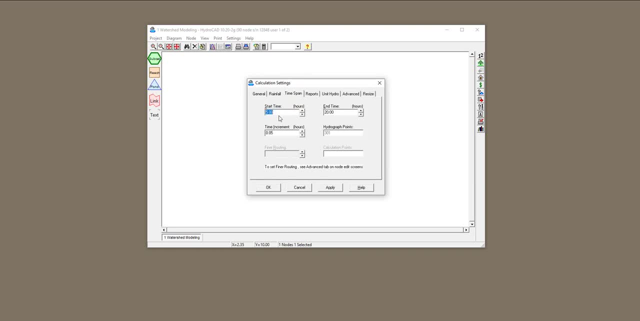 This is how we want our hydrograph to be modeled. Currently, by default, it's from five to 20.. We can change it later, but for now I'm going to keep it like this And the calculation time intervals right now is 0.05 hours. 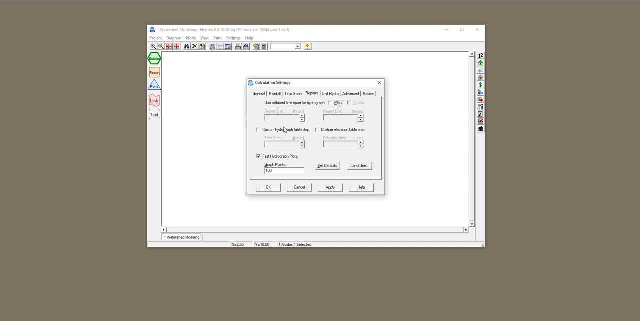 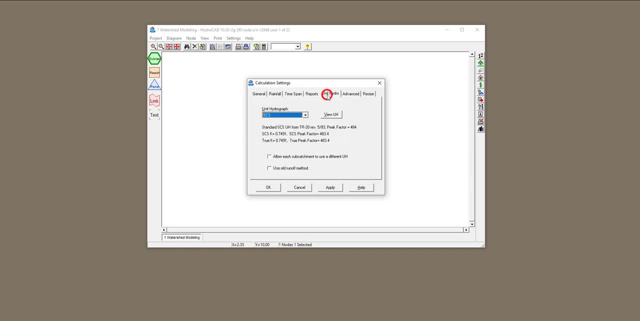 and what should not be included. Next tab is about the unit hydrograph. The unit hydrograph is a way that you can convert the depth of rainfall excess into a hydrograph at the outlet of your watershed. By default, it is the SCS unit hydrograph method. 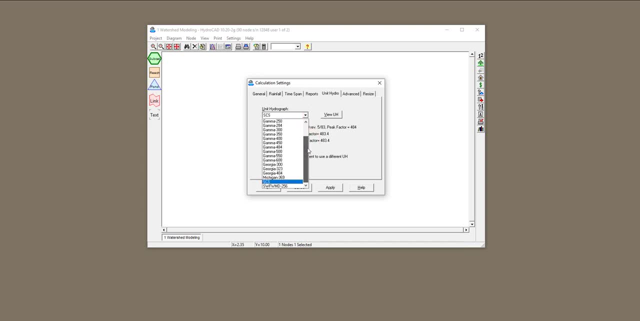 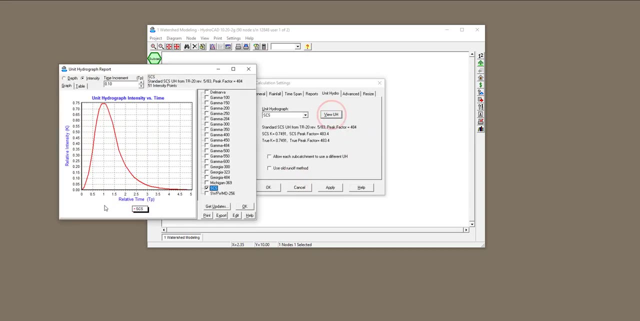 However, you can change this. You can change this to any other method that is available over here. I'm going to keep it as SCS hydrograph And when you click on view you will see the SCS unit hydrograph over here. 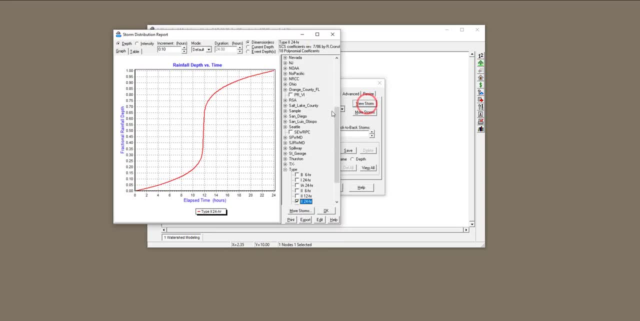 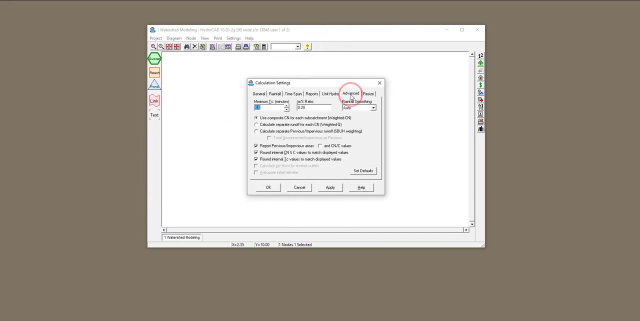 Similarly for rainfall. if you click on view storm, it will show you the 24 hour storm type two like this: And this is the value, incremental value for a fraction of rainfall: depth: Perfect. And then there is advanced that you can set a minimum time. 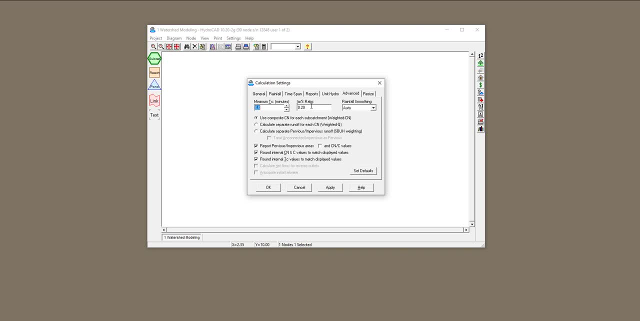 of concentration that I will be talking about And this is the initial abstraction coefficient which essentially is telling you right now. the initial abstraction, which is initial infiltration, depression storage and also interception, is only 20% of capital S or the maximum watershed storage. 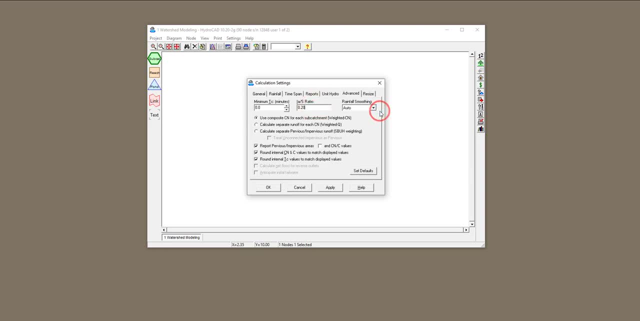 I'm going to keep it as 20%, but note that in some references this value could be 5% or 10%. So you are you can change this value too. All right, So I have set the rainfall and all the other variables. 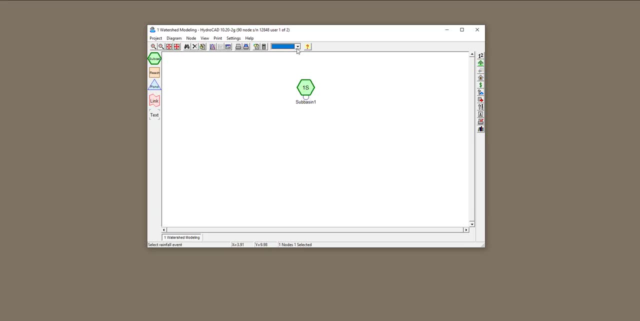 correctly. I'm going to click Okay, Now the watershed is ready. Actually, let's go back here and go back to rainfall. The depth is over here. You can name this depth as well. I'm going to name this step as scenario one, S one. 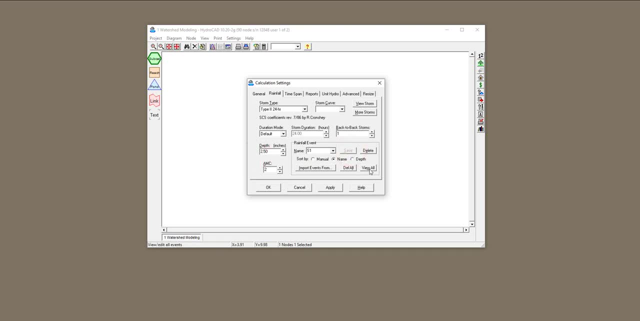 Okay. So and then click on save. So when you save it, when you click on view all, you can see the scenario that I have created over here. Let's create another scenario. Let's say that I want to have the depth of this time. 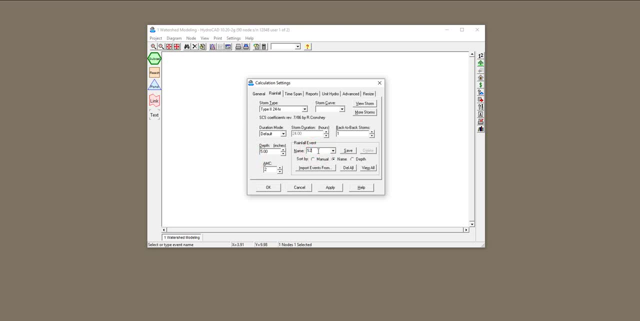 five inches, And this would be my scenario number two and I'm going to save it. So when you click on view all, you have two scenarios created. One has the depth of 2.5, the other one twice that, five inches. 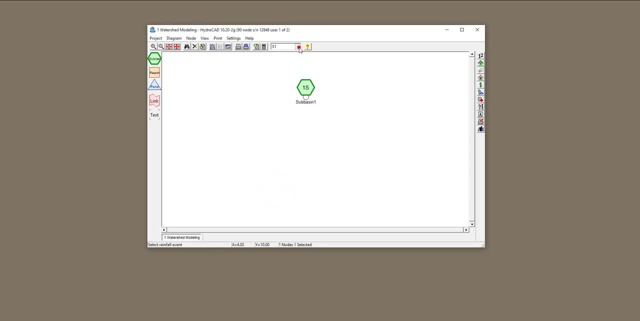 Okay, And now let's click. Okay, Now you will see over here you can switch between two different scenarios that you have. I'm going to click on scenario one And now, if you double click on this sub basin, you will see that the model automatically is going to create a. 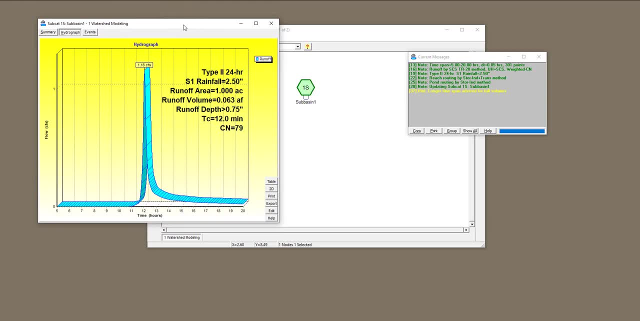 hydrograph for you. So the hydrologic modeling is done and it has created this hydrograph for you. The hydrograph is all over here And right now you are seeing a 3D version of this. If you want to see a 2D hydrograph, 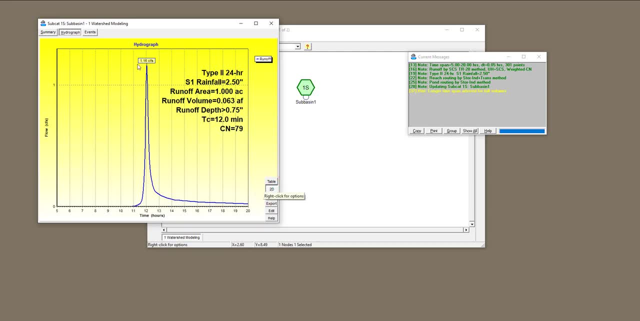 you can click on 2D and it will give you the 2D hydrograph, which has the peak of 1.6 CFS. All right, And it gives you some general information about your watershed and the runoff generated over here. 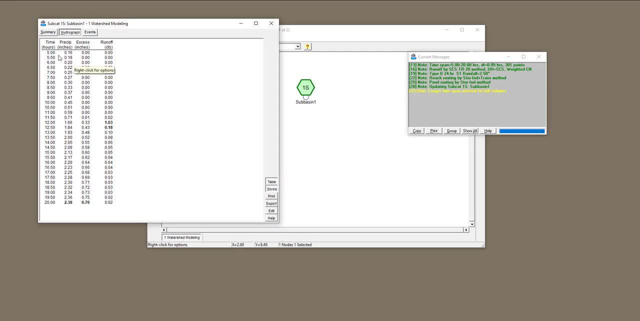 Okay, You can also see this hydrograph in form of a table. right now, you can see that the table is every half an hour. right, What if? but if you remember the calculate the time, the time stamp was not half an hour. 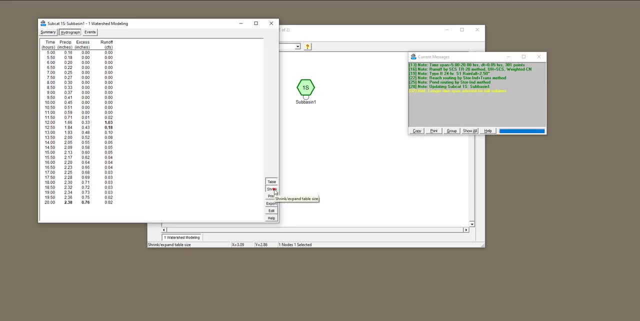 That's why, because the shrink button is on. If I turn this off now, you can see that the time span is different for unit hydrograph. Okay, This is just to save some time. And now, if you take a look at the values over here, 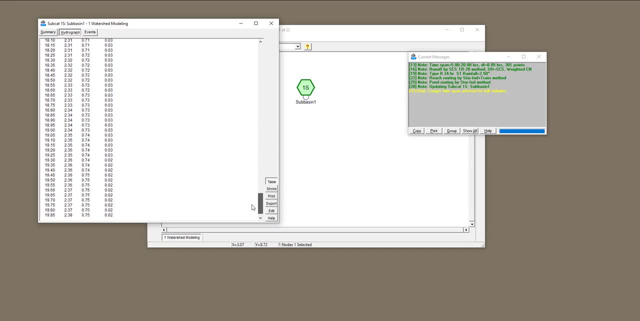 you will see that there are some values that are written essentially in bold, like this. Let me scroll down again These bold values. these represents the maximum or peak values. So if I want to show you this is if I click on the hydrograph, and then I want to show this. 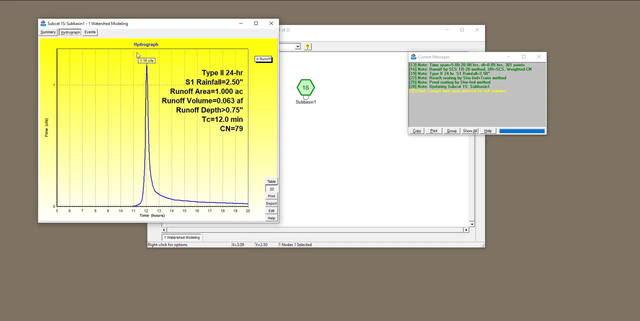 this would be the peak value of the hydrograph. that was written in bold and the table that I had. Okay, And obviously you can export this table into different folders that you have And if you want to change something, you can click on edit and you can change the area. 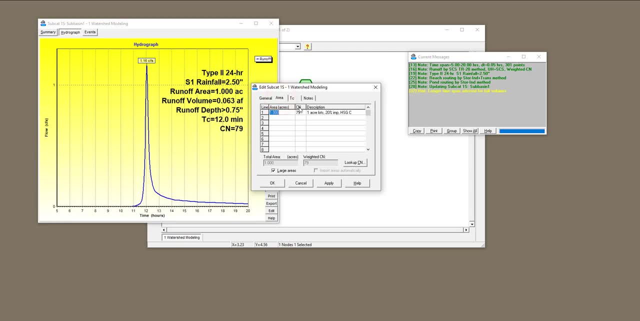 the curve number, the time of concentration. Let's say that we want to change the curve number, double click on it And instead of having a hydrologic soil group of C, I'm going to have the hydrologic soil group of D. 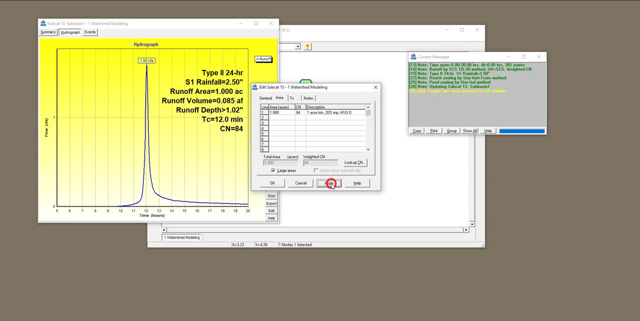 I'm going to double click on that This is changed. I'm going to click apply and you can see that as I clicked apply, this number changed. Perfect, And the curve number obviously has changed too. Okay, The other thing that you need to be careful when you're doing: 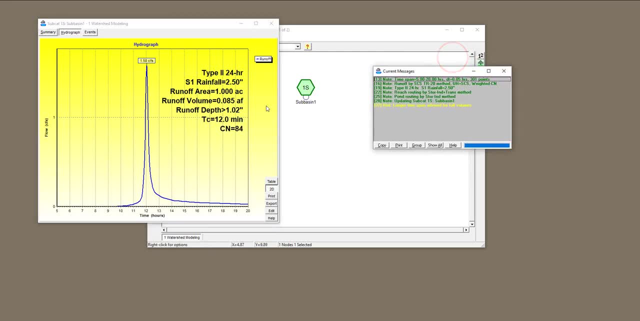 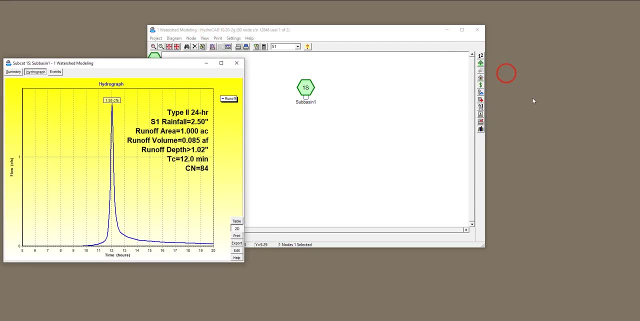 your simulations are the messages that you get, So the messages that you. let me reorient over here. sometimes you will see that this message box goes away. So if this goes away, you can click on this view all and the message box will show again. 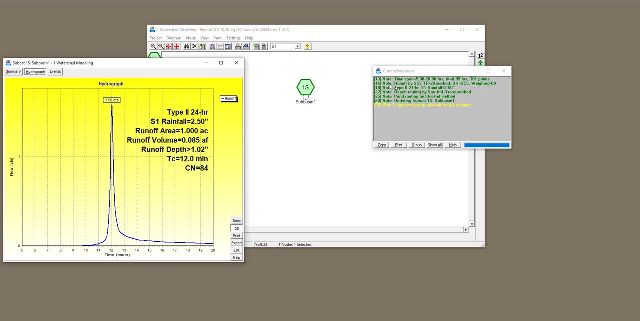 Okay, There are notes. everything that is in green There are just notes to you and it's okay. Hints are in yellow and warnings are in red. You do not want to have warnings. Hints are just trying to help you. give you hints to. 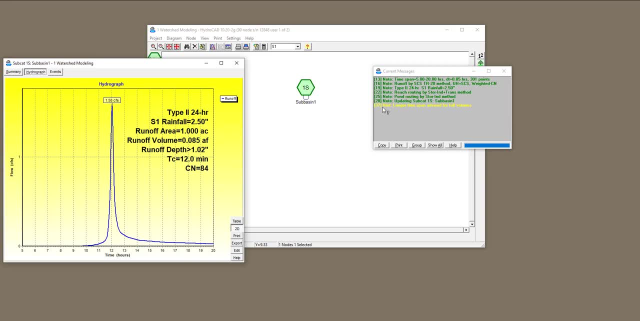 make your simulation better, or maybe visualization. For example, take a look at this: hints number 37. It says longer time span advised for full volumes. What does that mean? Take a look at the hydrograph over here. You can see that at the end of the hydrograph. 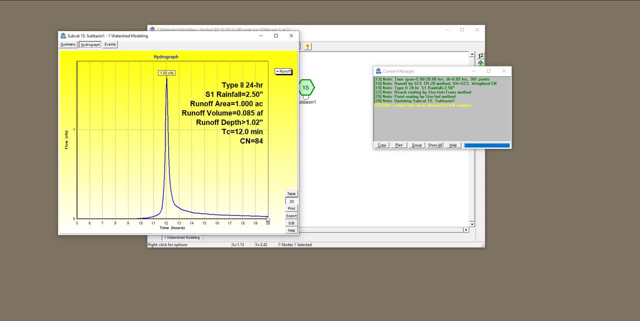 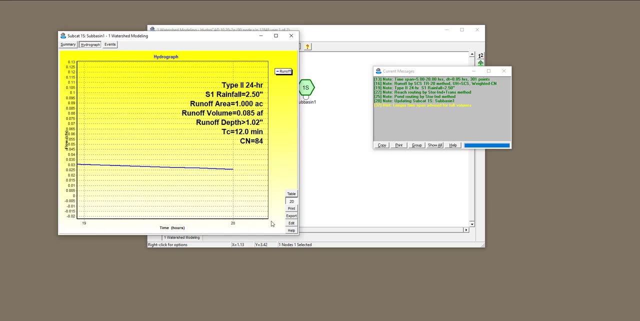 when the hour at our 20, the hydrograph does not have the value of zero, So I want to zoom in. If you want to zoom in, you just need to create a box over here from like this: So this is the zoom there. 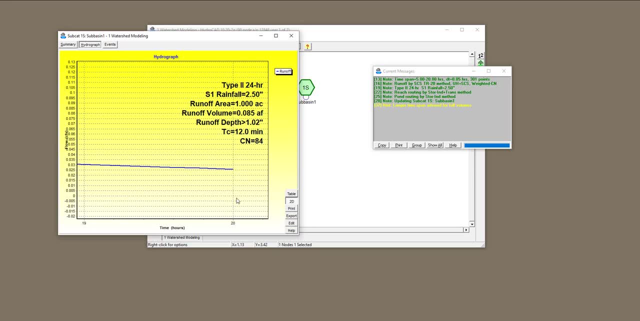 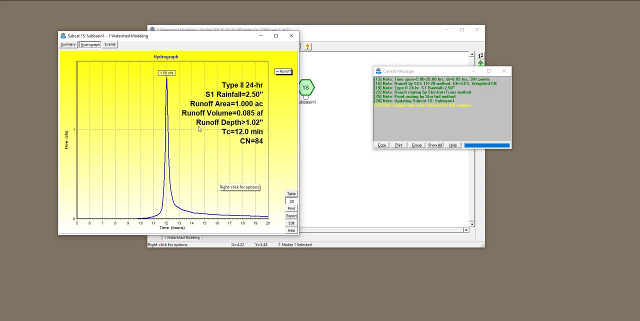 Admin, at 20 hours the value of hydrograph is not zero, right, And that's the error over here. It advises us to increase the hydrograph duration, So I'm going to create a box at the opposite direction, coming from the right bottom corner to to zoom out over here. 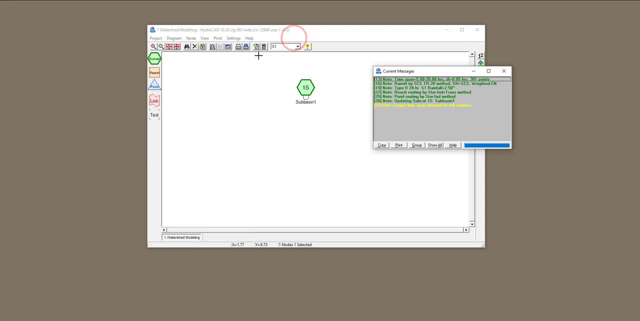 Okay, now let's close this and I'm going to click on this calculation settings right now. in the time span, You can see that my time span is from our five to our 20.. I'm going to change this to our 24.. 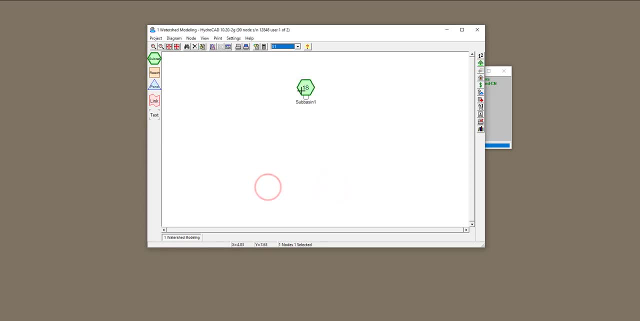 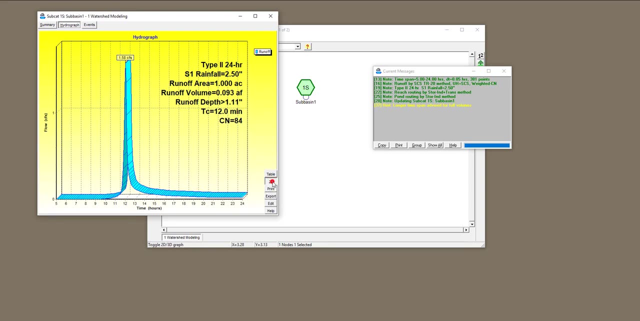 Okay, And then click apply and okay, And then double click on the sub basin. Now you can see that it still gives us that hints, because if I make it 2D and zoom in here again, still it's very close to zero. 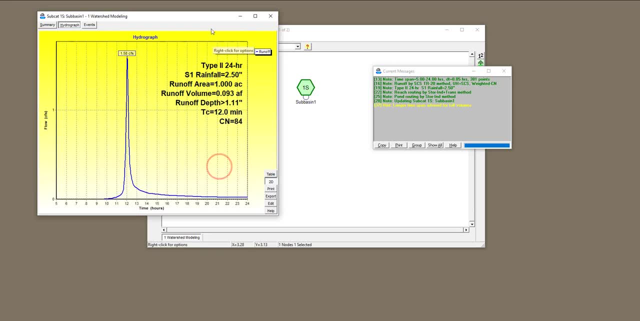 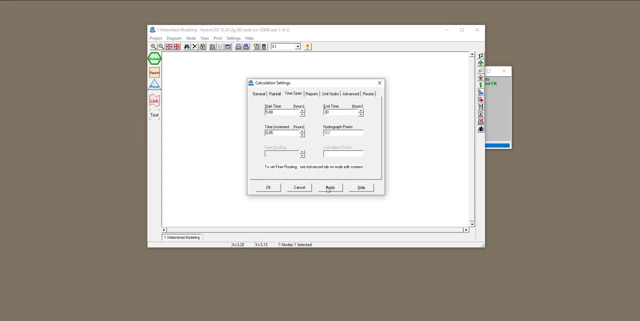 but it's not zero. So let's do this again. Zoom back, close this. going to calculation time span. I'm going to change it to 30 this time and then apply an okay Double click on your sub basin. Perfect. 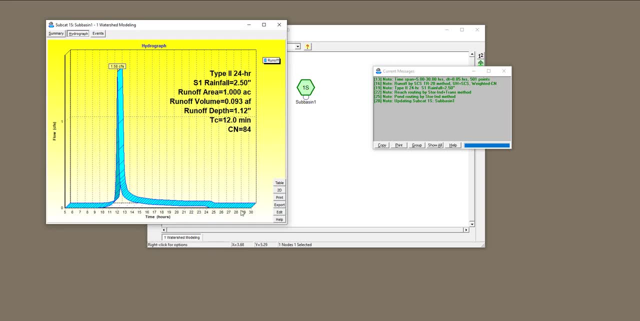 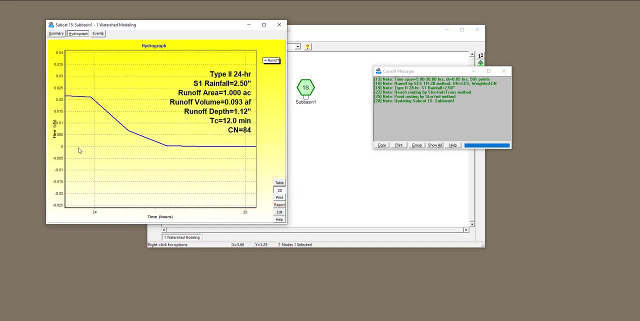 Right now you can see the hint went away and the hydrograph is equal to zero. after this point over here that I'm going to zoom in, There we go. You can see that it hits zero at this point, Perfect, Okay, so now, at any point. 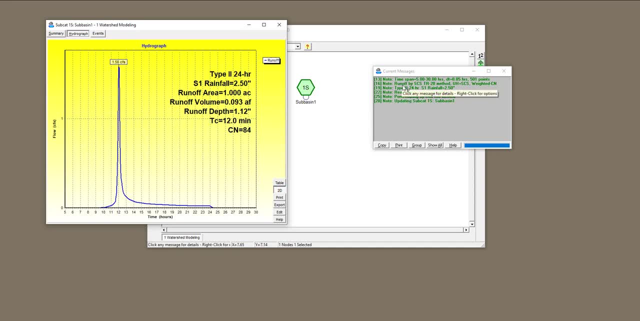 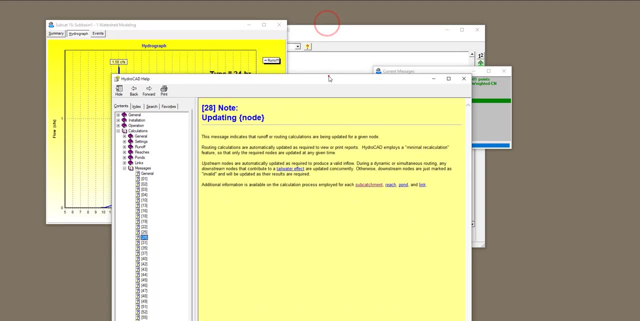 if you want to learn more about any of these warnings or hints or notes, you can click on these and it will open up for you the document for hydro cat that talks about that specific notes that you wanted to learn more about. Okay, I'm going to close that. 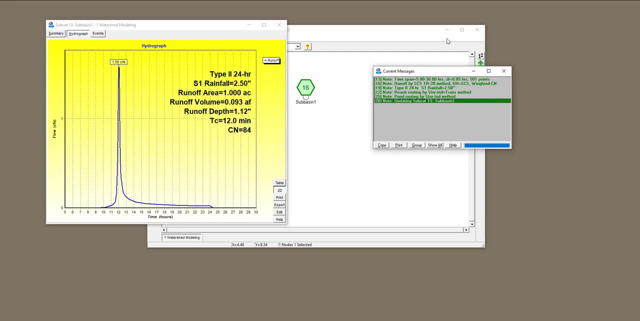 So this was your first tutorial, Very simple tutorial, Of how to use hydro cat for watershed modeling. Now, in the next tutorial, we are going to make this a little bit more complicated. What if we have multiple storms, and what if we have different values of curve number within the watershed, and so on and so forth, and do a little bit more complex watershed modeling. 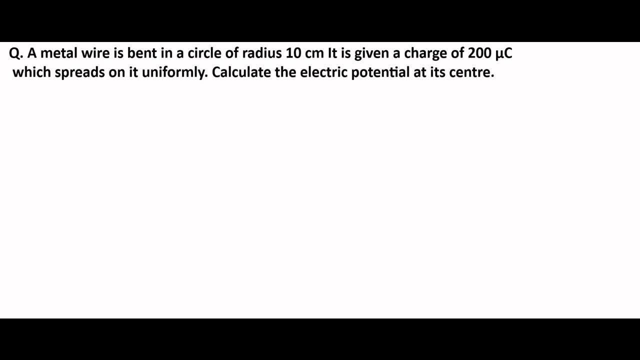 So here is another question on electric potential. So it is given that a metal wire is bent into a circle of radius 10 centimeter. It is given a charge of 200 microcoulomb which spreads out on it uniformly. Calculate the electric potential at its center. 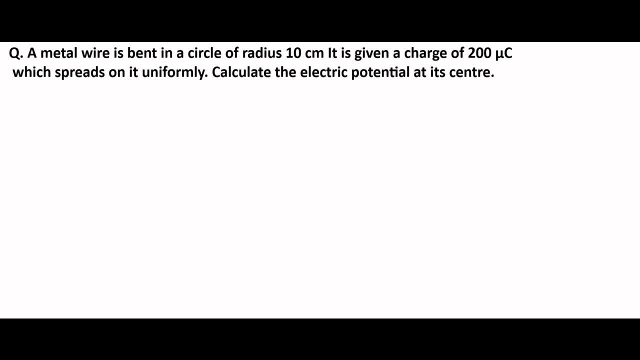 Okay. So here it is. given that we have a metal wire which is bent in the form of a circle, Okay, It has a total of 200 microcoulomb of charge which is uniformly spread. Okay, It is spread uniformly.